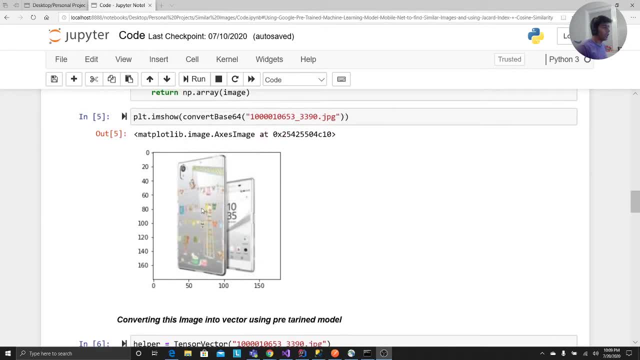 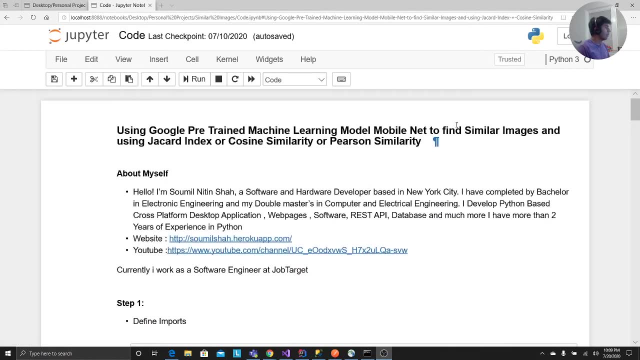 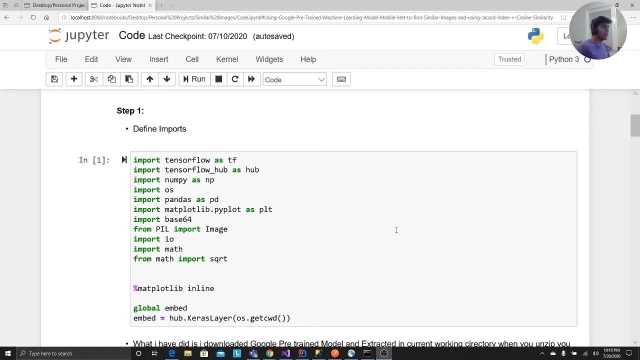 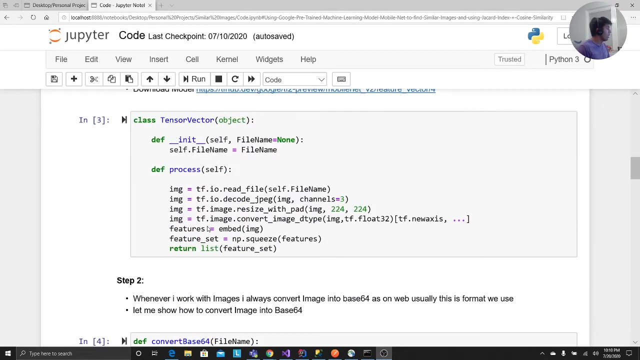 Like it's a mobile phone, right? So we need to apply some kind of algorithm, right? So TensorFlow Hub provides a pre-trained machine learning model. So I downloaded one of the model called MobileNet V2, which is basically an embedding- basically embedding- model. Basically, you provide an image and it basically outputs a vector of an image. So basically, when you have a vectors or an array of numbers, you can apply some mathematical equations. For example, one of the simple way to say that: 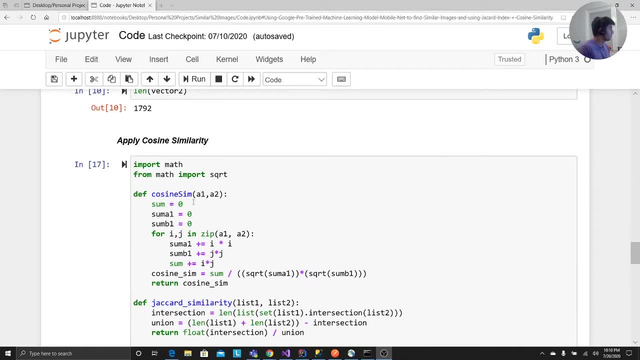 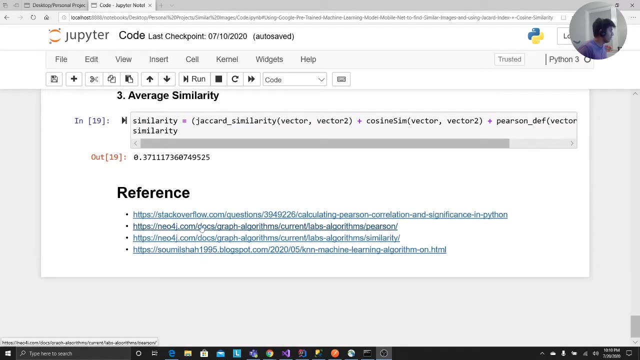 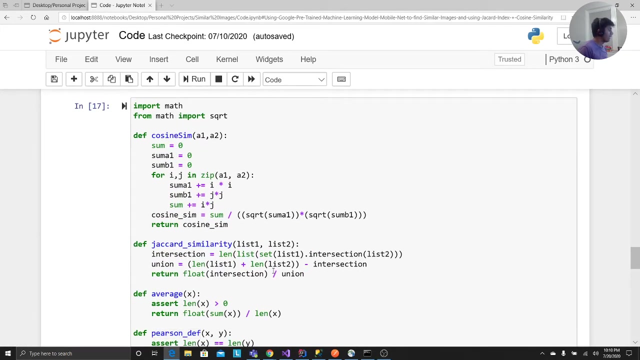 how similar this two images are is apply cosine similarity. Another algorithm that you might think is basically Jacquard index or Jacquard similarity. So if you are interested more in knowing about these kind of algorithms, I do have the links here in the description, in the reference section, where you can go and read more. OK, So let me just make it quick, OK. So the second algorithm I just said is a Jacquard index, So, which also tells you how similar two items are. right. After that we have 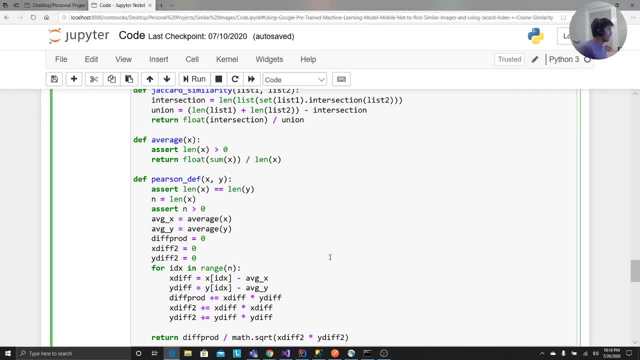 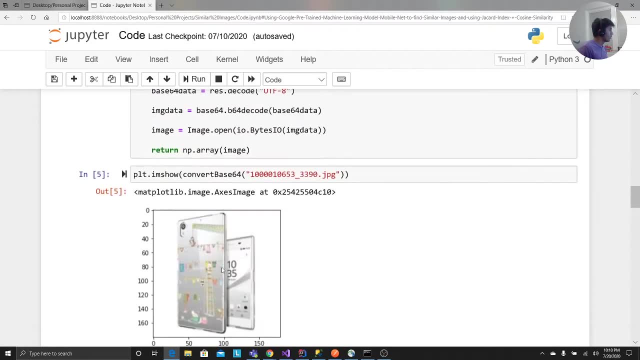 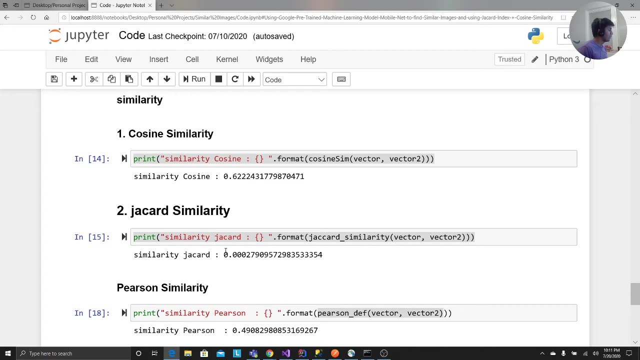 something called Pearson coefficient, which is again a similarity algorithm, and then then you can also compute Euclidean distances. so, based on cosine similarity, this image and this image, Cosine similarity says that is 62% similar. Jacquard similarity or Jacquard index, gives the number of 0.002.. 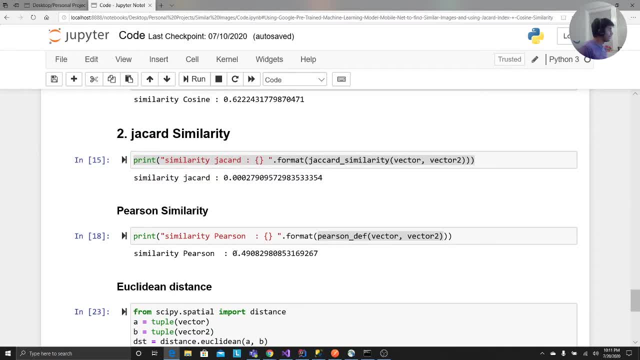 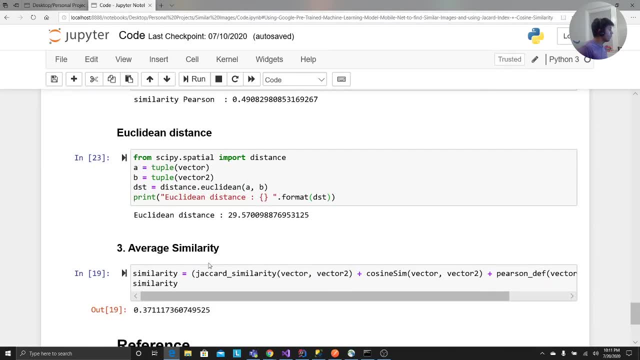 Pearson similarity says 0.49%. Euclidean distance is about 29% between these two vectors. so and if you want to combine all of these algorithm, what you can do is you can apply all the similarity algorithms and take an average value. so in this, 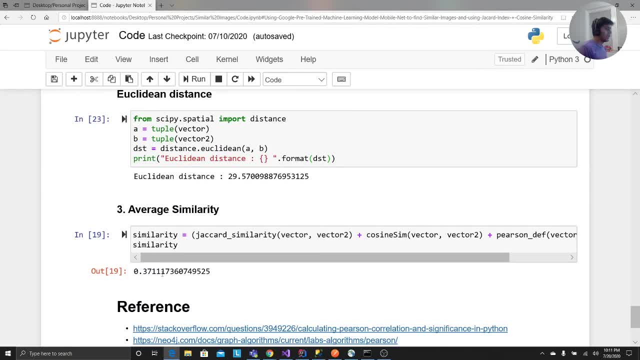 case. if you do that way, the average similarity of the images is 37%. so this also depends on highly of what kind of model you are using, because based on the model, you are gonna get the vectors right. so choosing the right model is very, very crucial in this. so I just picked up a random model like the one 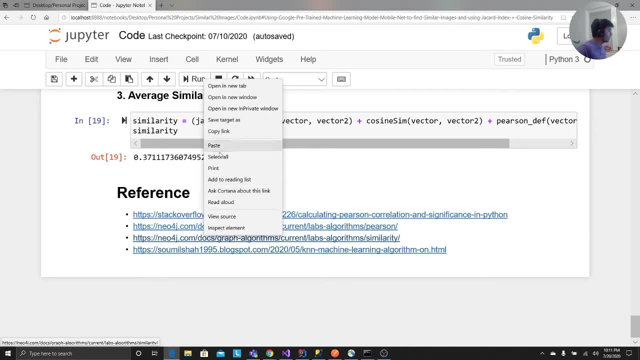 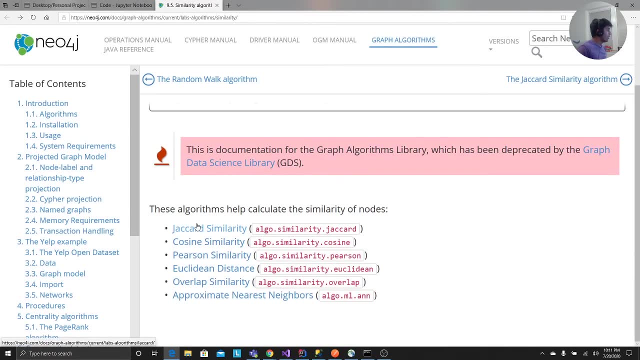 they had. if you are interested and if you want to read more, I want to show you a link that I have it in the reference. I would leave everything in the description so you can read it. so jacquard similarity- cosine similarity- Pearson similarity Euclidean distance: overlap similarity- approximate nearest.